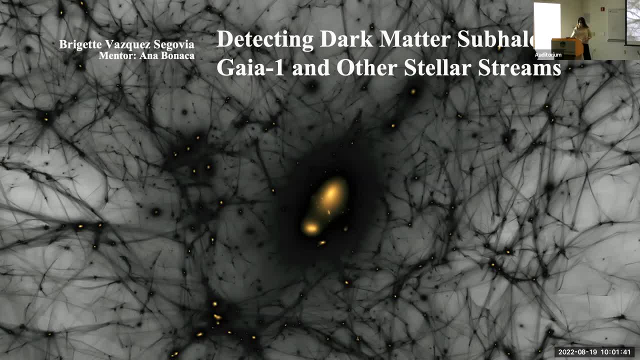 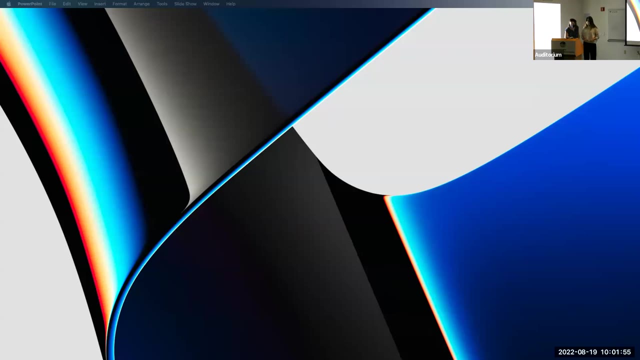 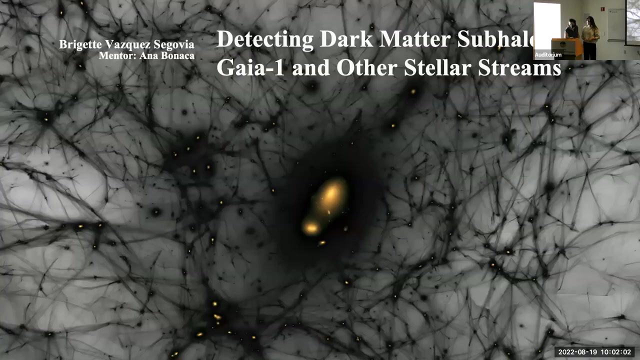 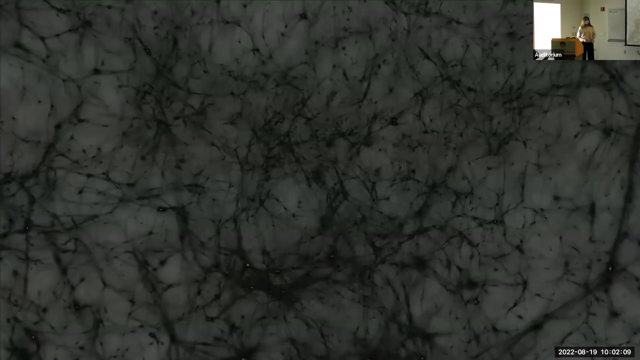 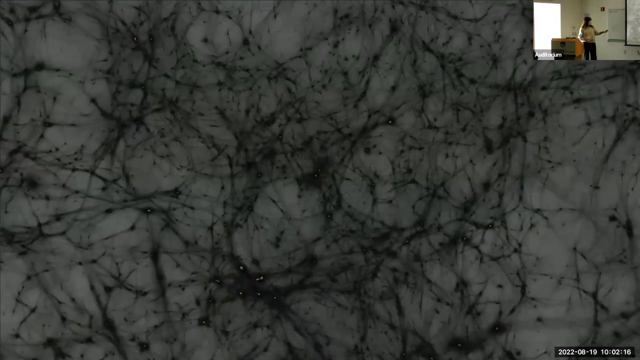 But how exactly is this dark matter halo formed? I think it's kind of Technical difficulties. One second, All right. So here I am showing a high resolution simulation provided by Ethan Nadler And, as you can see, here in dark, in black, we see that dark matter starts off being pretty hollow. 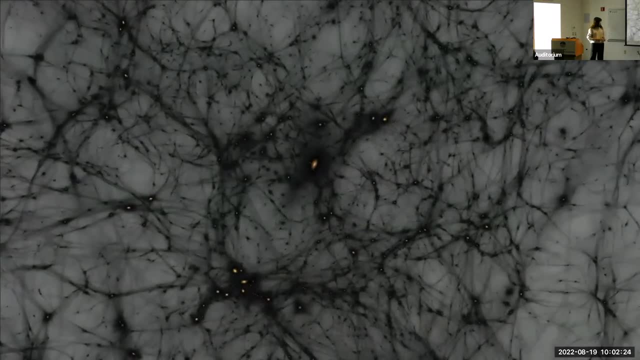 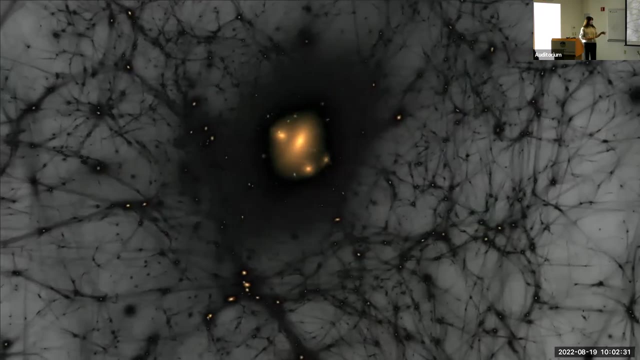 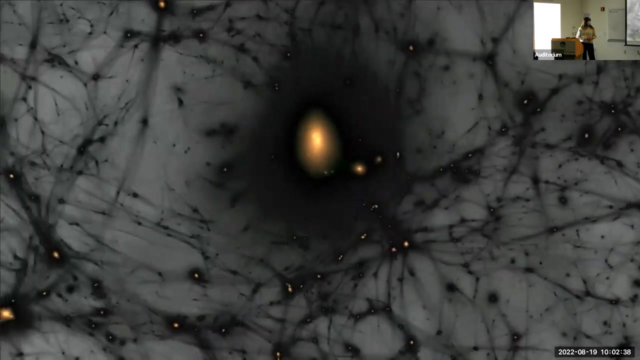 It starts off being homogenous. We see these filaments of dark matter and in yellow we see the galaxies. Right now you will see a zoom in of the Milky Way with its large Magellanic cloud, And once again we see this dark matter halo that sort of surrounds the Milky Way. 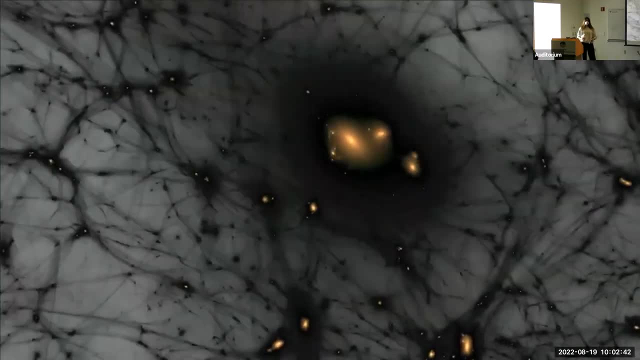 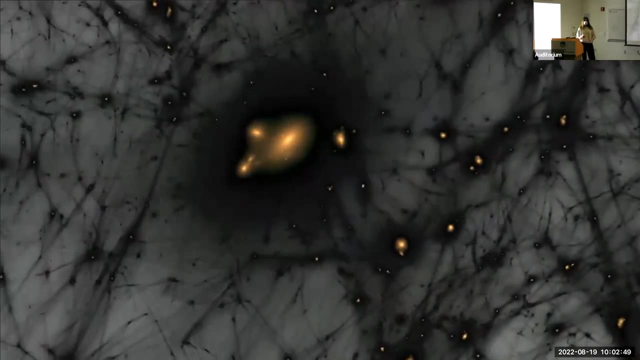 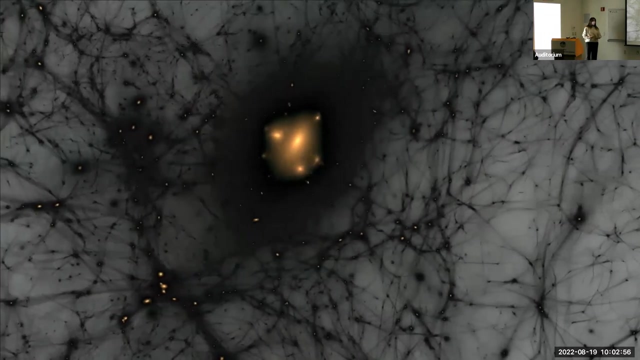 This dark matter halo is made out of thousands of subhalos, which are also made out of dark matter particles, And, as you can see here inside the halo, there are not many stars that live in there, Making it difficult for us to sort of even think about what the model, what the best model for this dark matter could be like. 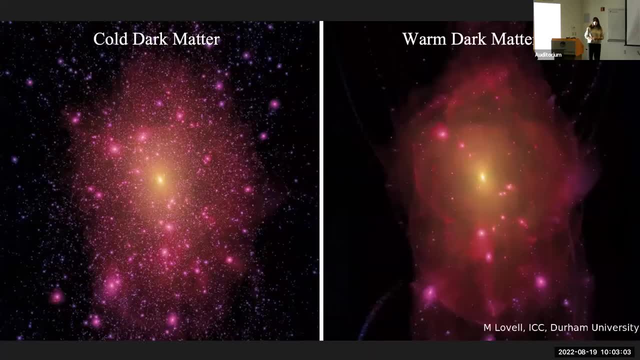 In the previous simulation, the representation of dark matter was more of a cold dark matter And, as you can see, there are many particles compared to the warm dark matter, which is another one of our models for what dark matter can possibly look like in our sky. 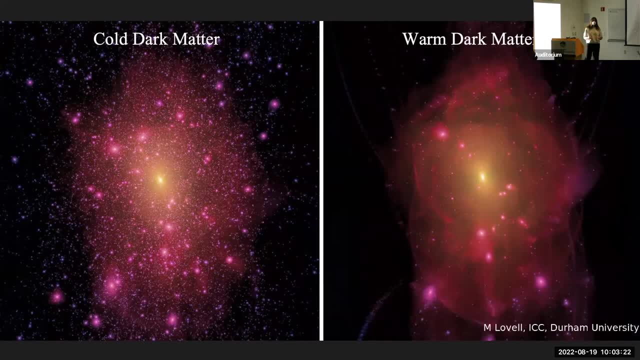 Both of these images show the same amount of mass in our sky for dark matter. However, as you can see, there is a clear distinction between cold dark matter and warm dark matter. One of the other main distinctions between these two models is that cold dark matter moves much more slower than warm dark matter, hence giving it its most famous name. 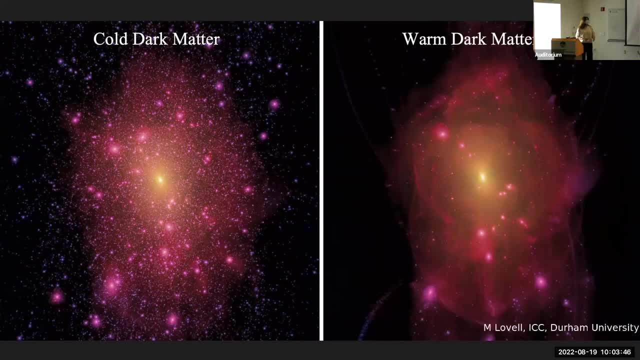 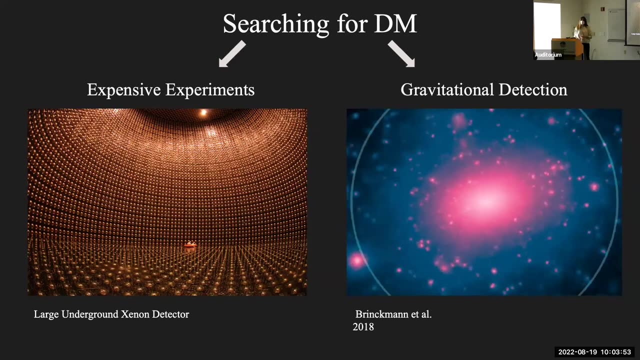 And in efforts to detect which model best fits our sky, scientists have used two main ways, which is through expensive experiments or through gravitational detection. In the expensive experiments wave here I am showing what the large underground xenon detector looks like And essentially here we would fill this tank up with xenon. 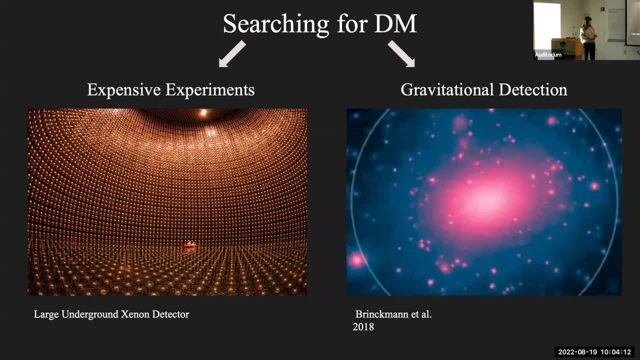 Xenon is a high mass and also a noble gas, So scientists believe that if anything as heavy as dark matter was to come in close contact with any of the atoms found inside this tank, one of these thousands of detectors will figure out that there is a perturbation going on. 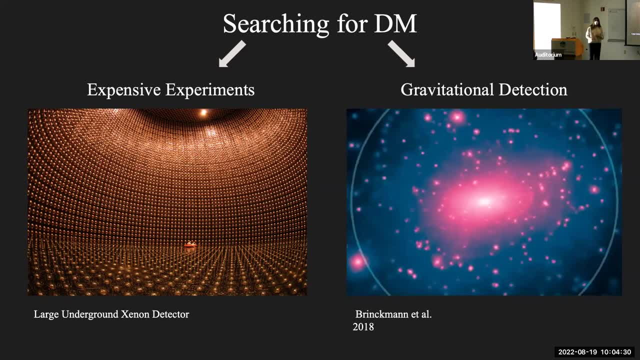 However, we have been heavily unsuccessful in finding dark matter in this way, So we have resorted to something more of a gravitational detection, which is obviously a more astronomical sort of scale. Here, once again, I am showing the dark matter subhalos that live inside this. 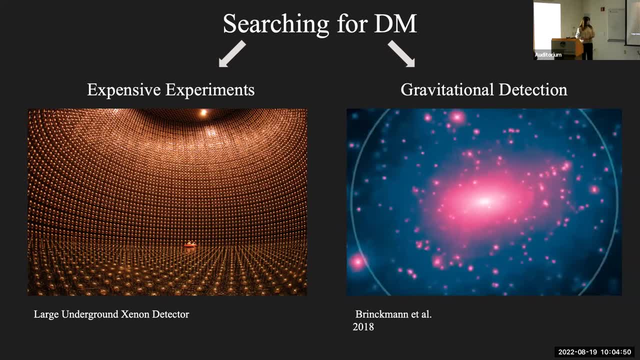 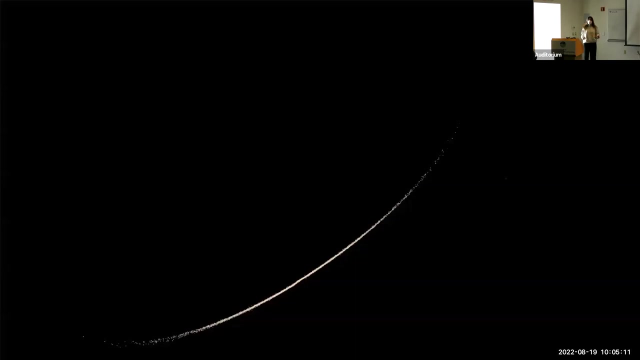 dark matter halo cloud And in the center, once again, there is a Milky Way. And one of the main ways that we have- Okay, I think it froze again, Okay, Okay, one of the main things that we have been using in order to sort of track where these dark matter subhalos lie in our sky. 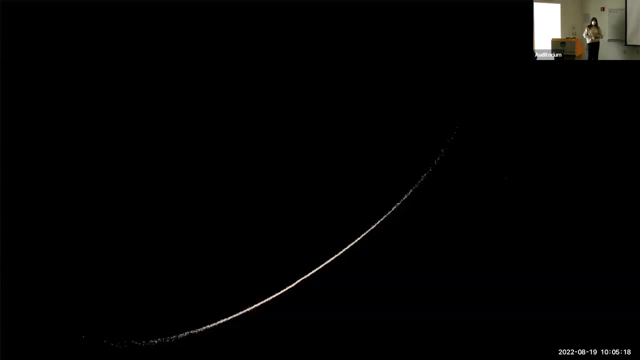 is through stellar streams. Stellar streams are these long ribbons of stars that form from globular clusters or four galaxies, through tidal disruptions And, as you can see here, we believe that if something as heavy as a dark matter, subhalo, was to come in close contact with the stellar stream, 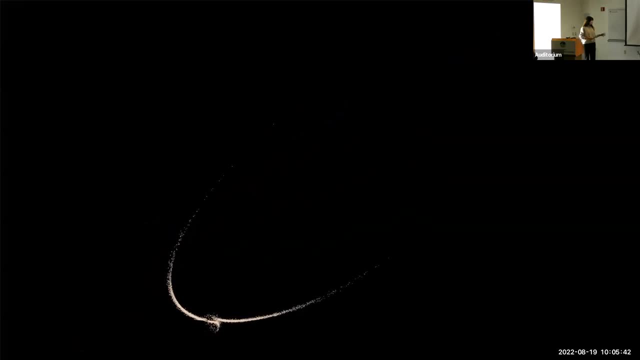 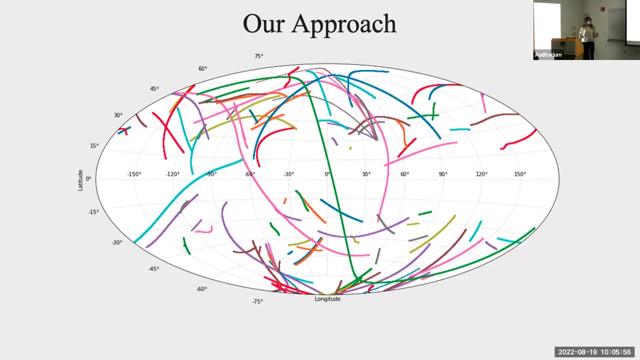 the stars in the stellar stream would suddenly become disrupted. They will shoot out in different ways, And this is something that we hope we can observe in our sky. So for our main approach of this project, we first started by looking at the 97 previously detected stellar streams. 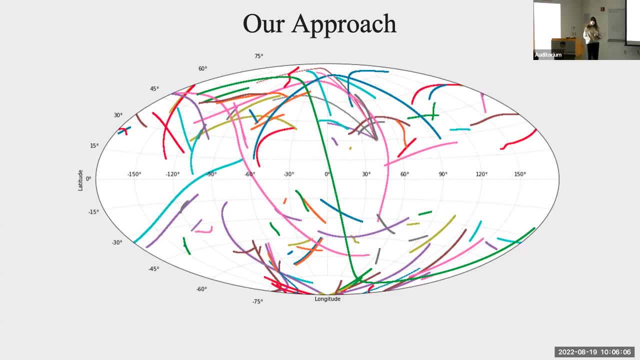 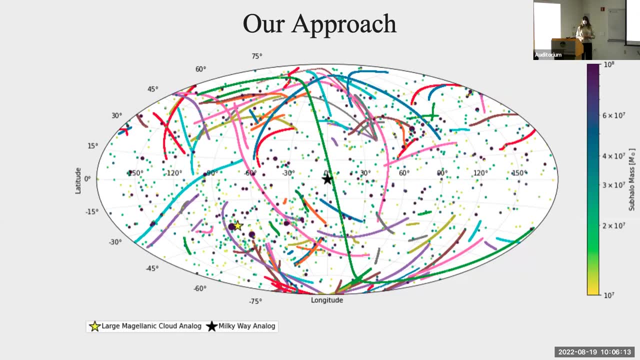 These 97 stellar streams were nicely concise in Cecilia Muthu's catalog that was published this year, And here I am plotting the simulation that I worked with for this summer. This simulation is of dark matter subhalos. It is a high resolution simulation that resolves subhalos to the mass of 10 to the 7 solar masses. 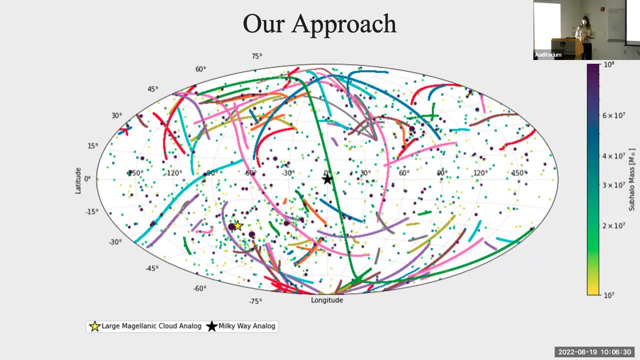 And, as you can see here, the distribution of these dark matter subhalos is not very homogenous. Here we see bigger and darker dots, meaning that these subhalos are more massive and they tend to be closer to something such as the Large Magellanic Sun. 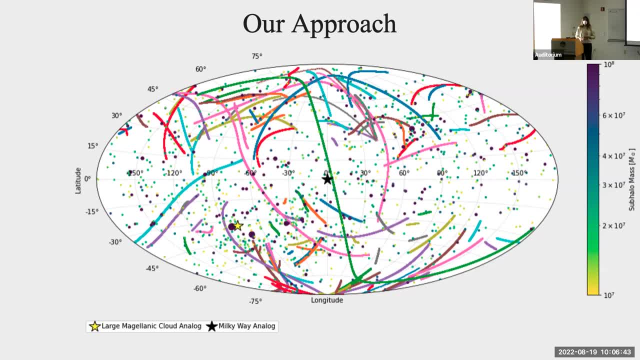 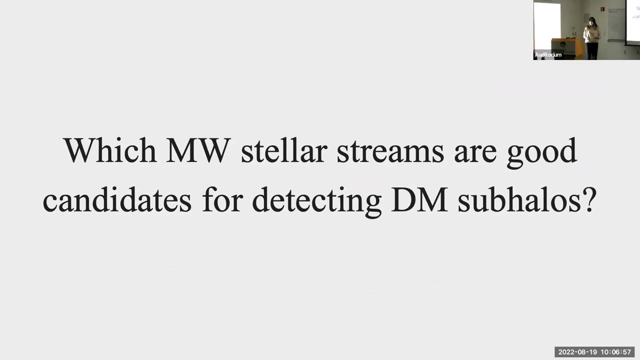 They tend to be closer to something such as the Large Magellanic Cloud Analog, mostly due to its gravitational bounds, And it's just a very heavy area in the sky. This drove us to the main goal for our project, which was to detect which Milky Way stellar streams were the best candidates for detecting these dark matter subhalos. 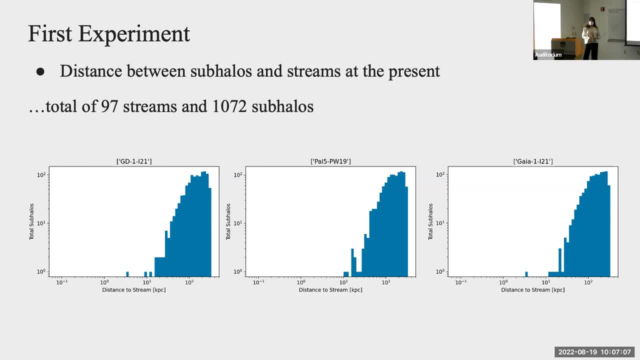 Our first experiment was to try to look at the distance between subhalos and streams. in the present There are a total of 97 streams and I was working with a total of 1,072 subhalos. Here I am showing three of the stellar streams found in the 97 stellar streams catalog. 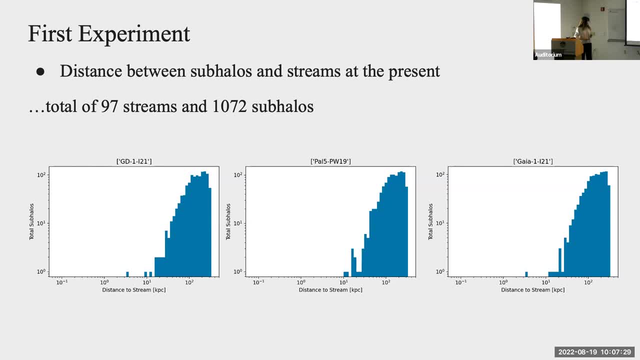 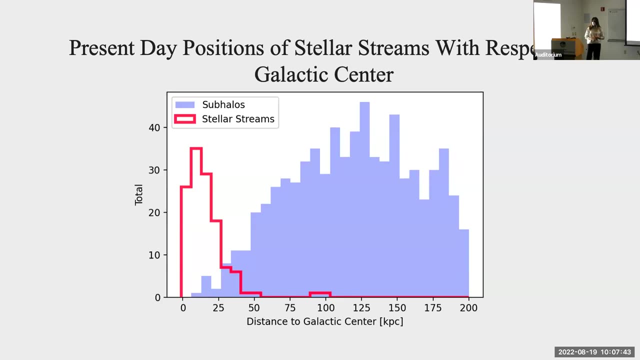 And, as you can see, most of the subhalos don't even surpass the 10 kiloparsecs distance between stream to subhalo. More specifically, we see that in the present-day positions of stellar streams with respect to the galactic center. 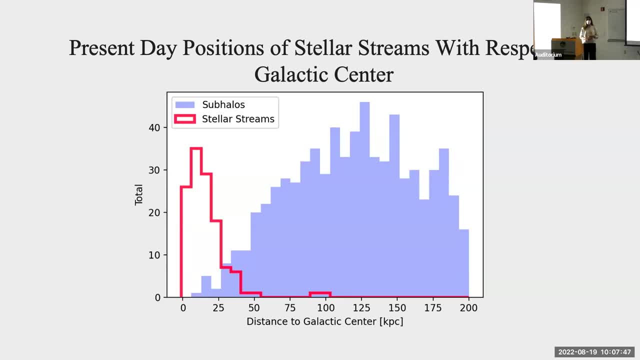 the stellar streams lie within 0 to about 20 kiloparsecs from our galactic center, compared to the subhalos, which extend all the way to 200 kiloparsecs and even further. This was sort of a problem for us. 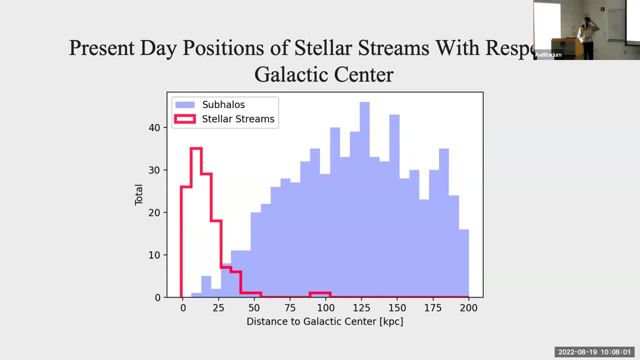 because it wasn't evident for us to make sure that any stellar stream would actually come in close contact with subhalos in the present. This created a shift in our project and we started thinking more about: well, if it doesn't happen in the present? 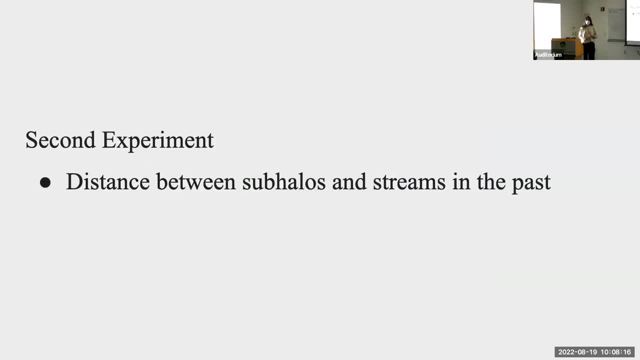 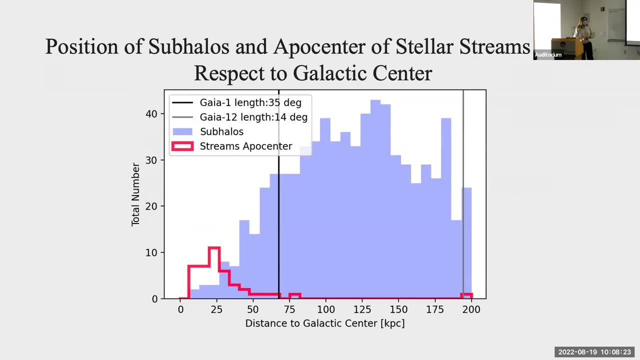 maybe it could have happened in the past. So we started looking at the distance between subhalos and streams in the past. Here I am plotting the position of subhalos and the epicenter of stellar streams with respect to the galactic center. 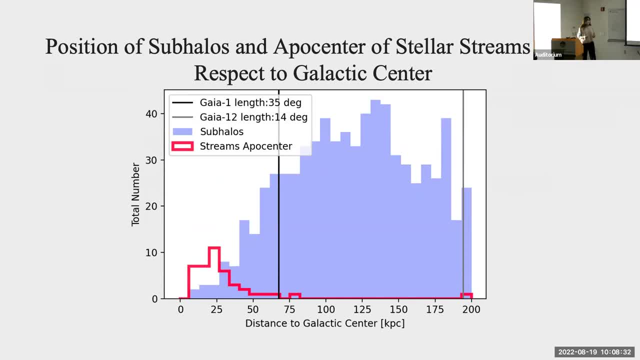 The epicenter is the furthest distance in orbit that a stellar stream can be with respect to the galactic center, And I have labeled two of the main stellar streams that I was considering Here. I have Gaia-1, which is the one that I actually ended up using. 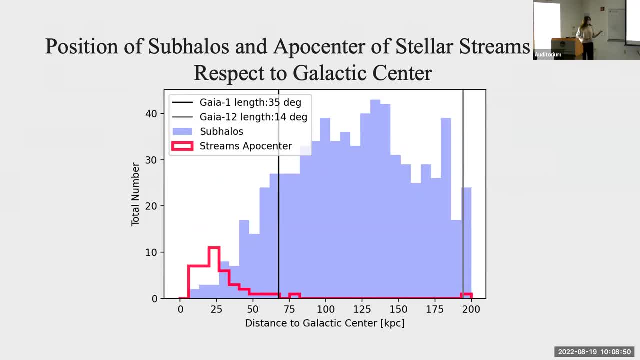 and I also labeled Gaia-12.. Although Gaia-12 has a large epicenter, we did not end up selecting it to be the main stellar stream to look at, simply because of its length of 14 degrees, compared to Gaia-1's of 35 degrees. 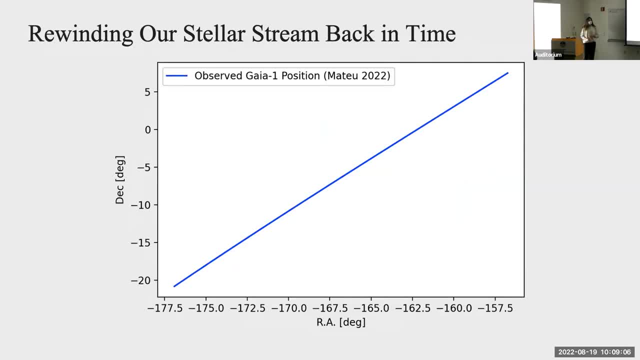 So, in order to get the position of the stellar stream in the past, we started this rewinding of time by taking the actual observed data presented in Cecilia Mathieu's paper. Then, using Malhan's paper, I was able to obtain the initial orbital position. 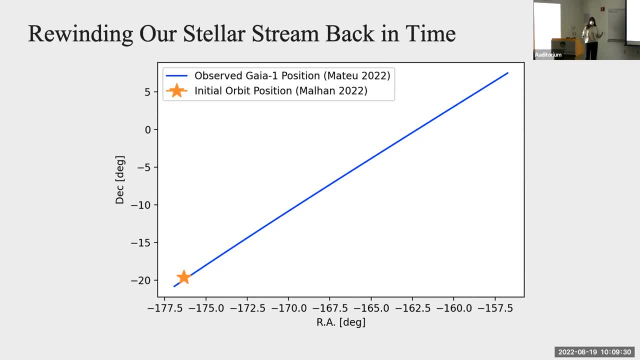 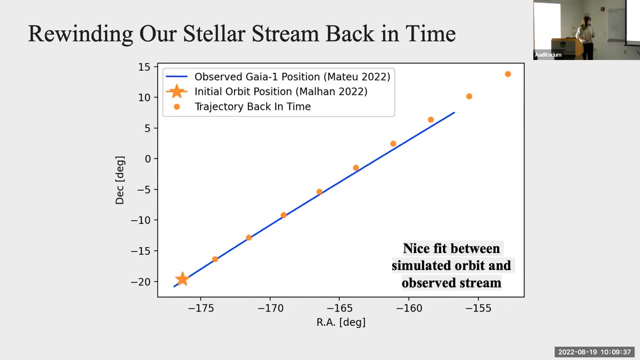 So Malhan's paper also provided me with the 3D position and the 3D velocity of the stellar stream, And using that I was able to map out certain checkpoints as to where this initial position could have been in the past. Here. 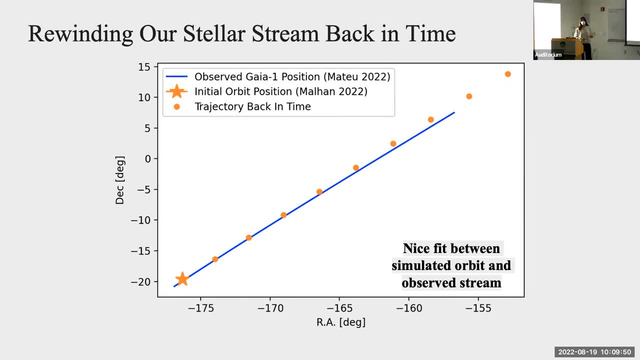 I have labeled different dots. Each are of a distance of one mega year going back in time And, as you can see, there is a very nice fit between the simulated orbit data, which is in orange, and the actual observed stream, which is very exciting for us. 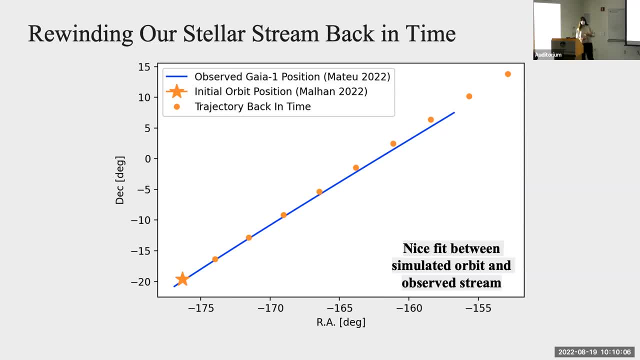 Keep in mind that this uh simulated data was actually done using the Milky Way's analog, so that from my simulation using the Milky Way's analog, um position and mass, So with this I was able to take nine checkpoints that sort of represented this stellar stream. 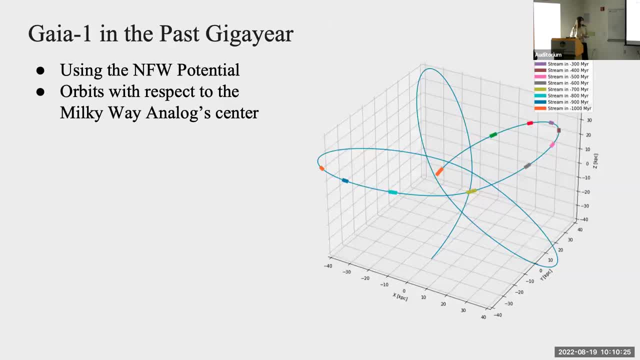 and track it even more back in time. So here I am showing how, using the Navarro-Frank white potential and the orbit with respect to the Milky Way's analog center, I was able to track back where Gaia-1 was found in the past. 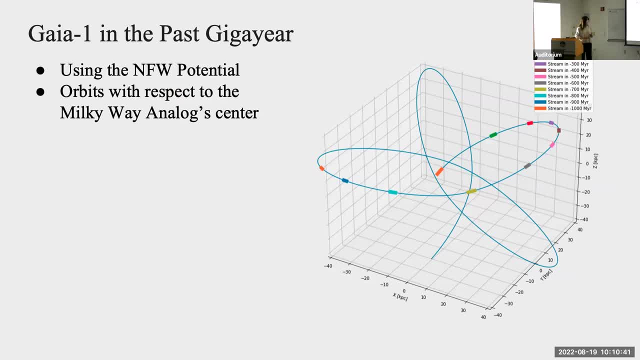 In light blue I am showing Gaia-1, which um over the span of three giga years, and in these little checkpoint boxes it's a separation of 100 mega years. Okay, um, I think uh. 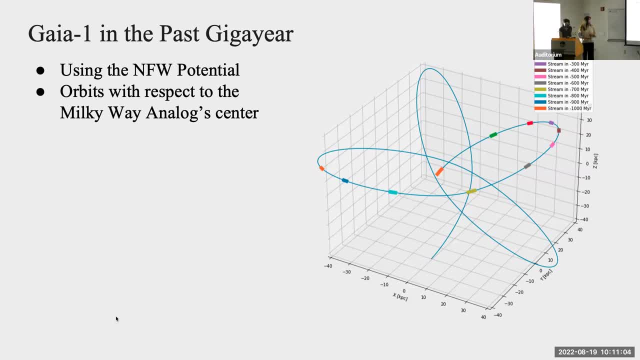 if you think of this, you can see that, compared to the one that I showed you in black, it's about a quarter of a trillion years ago. All right, I am ready to continue. Um, so we ended up doing the exact same thing for the 1072 subhalos. 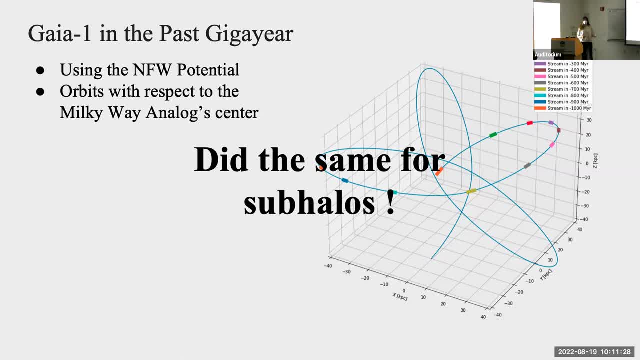 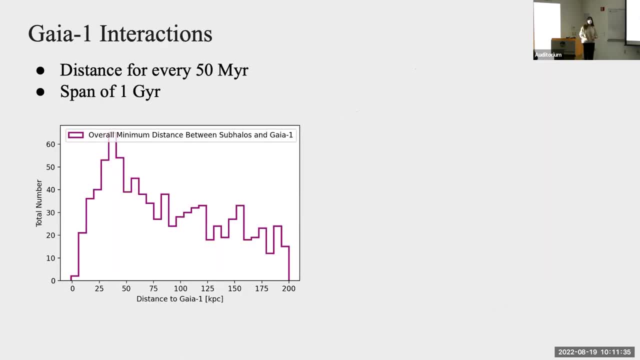 The main difference with working with subhalos was that I was just able to treat it as a single particle rather than in a segment of an orbit. So over the span of one giga year, I created a checkpoint for every 50 mega years. 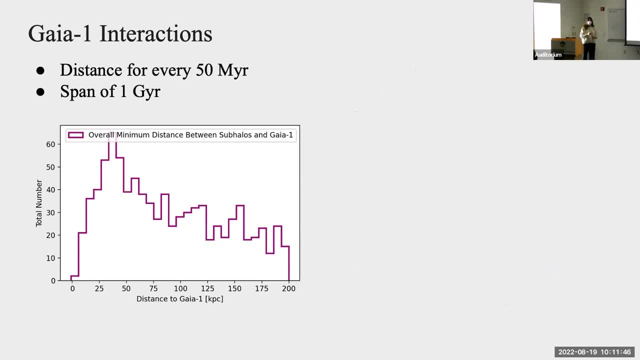 and calculated the distance between Gaia-1 and all of the subhalos. I determined the shortest distance at that specific time And over the span of this giga year. here I am showing the overall minimum distance between subhalos and Gaia-1.. 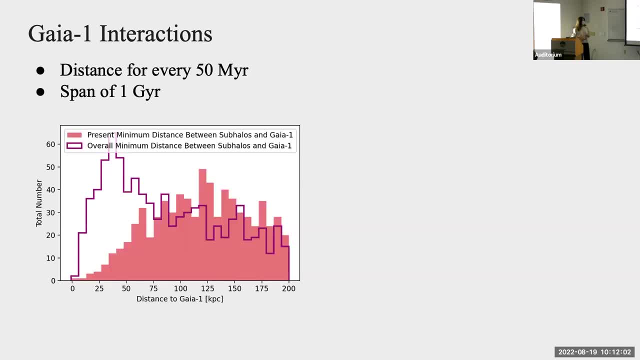 And it was very exciting for us to see that it was completely different than if we were to just sort of find the minimum distance at the present. So here once again in the present, in this brownish color, I am showing the distance between the subhalos to Gaia-1.. 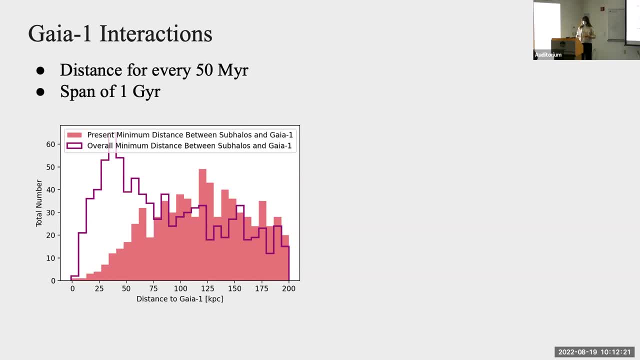 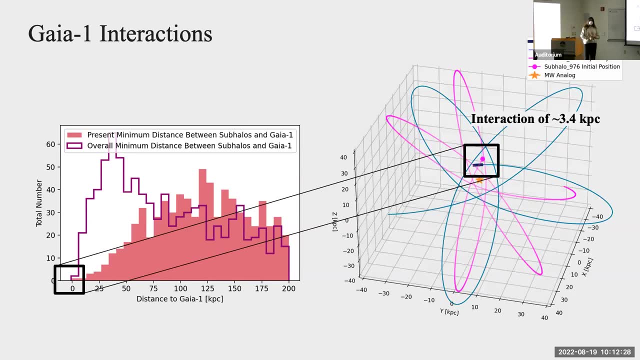 And this big shift just caused a great excitement for us. And here I am showing the nearest interaction between the subhalos and Gaia-1. Which would actually be happening in the present of 3.4 kiloparsecs. Once again, I'm showing the orbit of Gaia-1 in light blue. 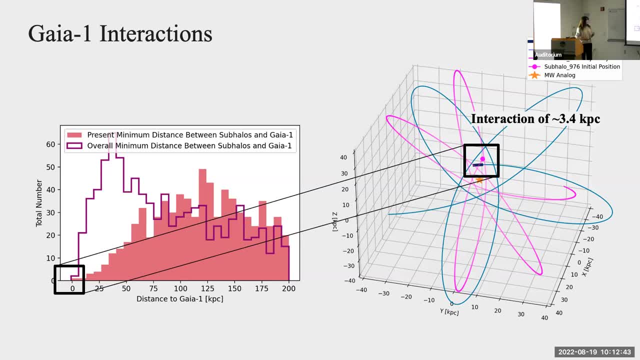 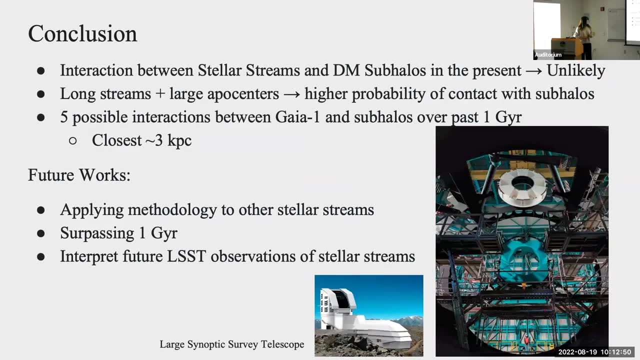 over the span of three giga years, And in magenta I am representing this subhalo that came in closest contact with Gaia-1.. Okay, so, in conclusion, we did find that the interaction between stellar streams and dark matter subhalos. 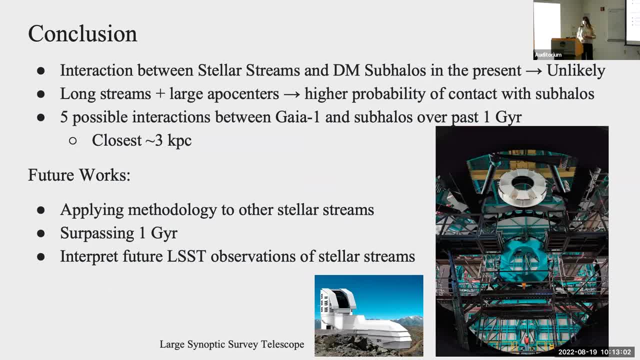 in the present is very similar. Okay, so in conclusion, we did find that the interaction between stellar streams and dark matter subhalos- in the present is very similar- is very unlikely. Long streams plus a large epicenter, however, can give us a higher probability. 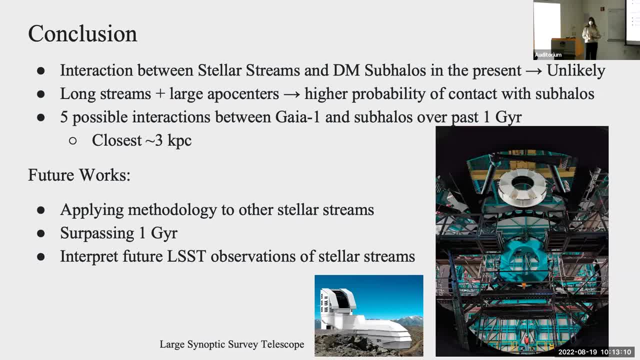 of having come in close contact with subhalos and interacting with them. There were a total of five possible interactions between Gaia-1 and the subhalos that I worked with over the past giga year, And the closest one being of approximately three kiloparsecs. 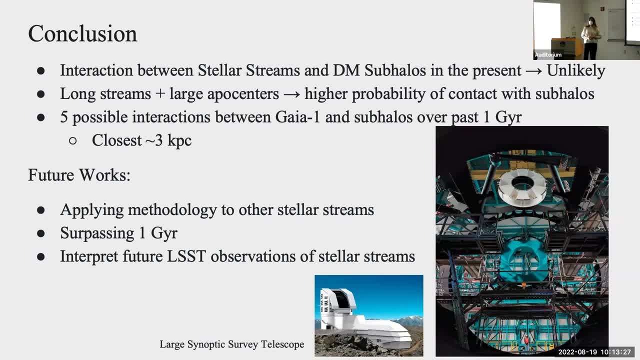 For future works. I hope to continue working with Annaponazza and applying this methodology to the remaining 96 stellar streams. We were also considering surpassing the one giga year bounds that I established, And all of this data can also help us interpret. 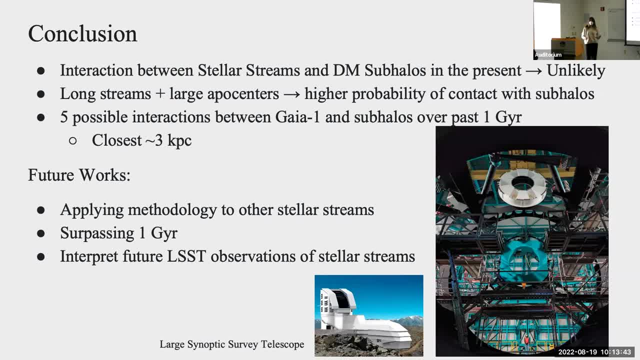 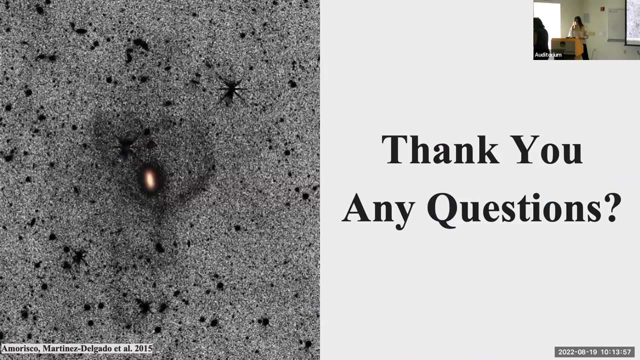 the future LSST observations of stellar streams, which is a telescope that we'll actually be launching next year, And without further ado. thank you so much, And if you have any questions, I will gladly answer them. Thank you, Excellent talk. 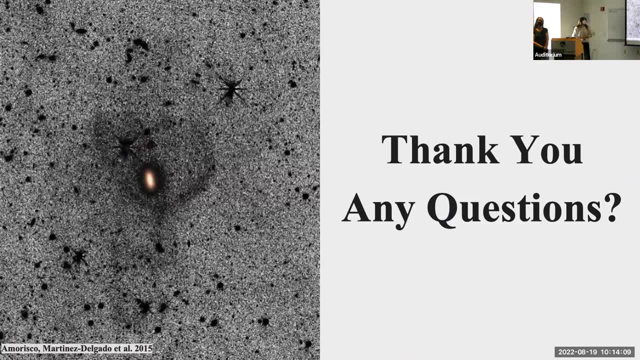 Thank you for dealing so wonderfully with all of the interactions. We have a question for Bridget in the back. Alicia, I have a hypothesis that the- Let me repeat the question- So do you have a hypothesis for how close the streams are in the present? 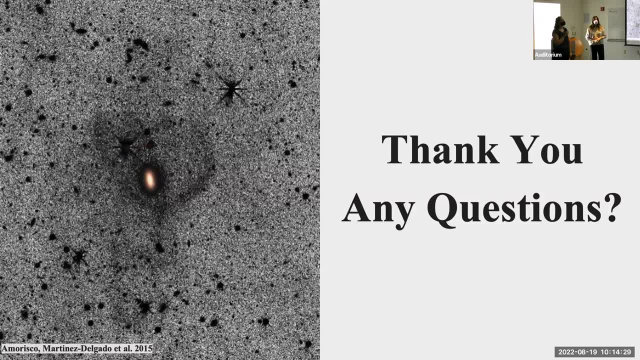 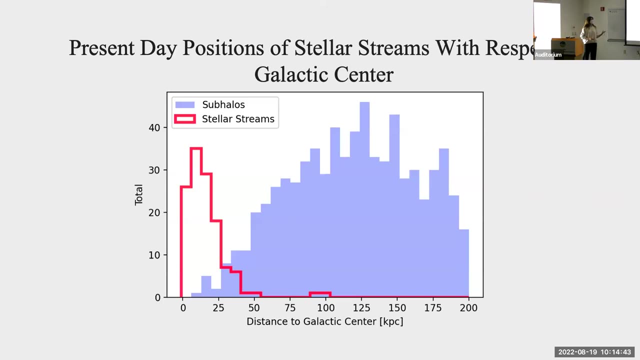 Before you started the project, and why Before you started the project? and why? why? yes, so we actually did not have a very specific number that we were thinking, but we did think that they would be a lot closer than expected. the okay. so we actually didn't really. 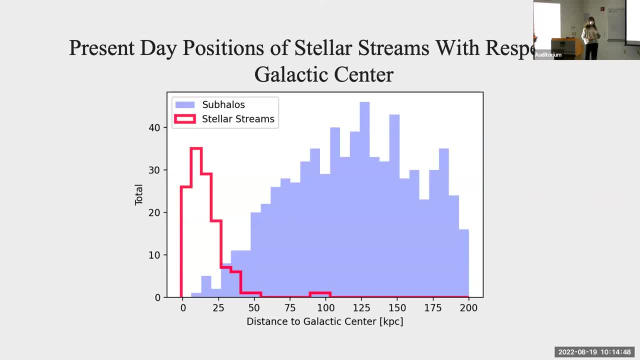 know that they would lie so close to the galactic center compared to the remaining um subhalos that we were working with until maybe even half in the program, and we were in total shock about this. and that's when we just try to like think of different ways that we can tackle this issue. 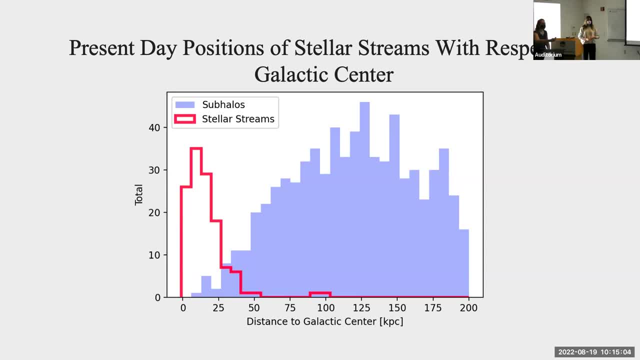 other questions. so you mentioned that you have five close interactions with Gaia-1 and subhalos. so was it with a similar kind of subhalo or like what was going on over there? um, yes, so we did have a total of five near interactions that we considered of less than. 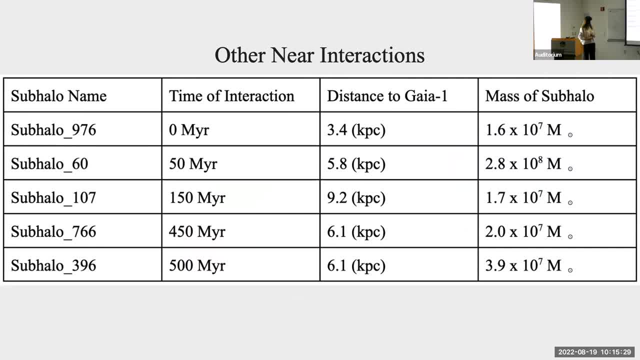 10 kiloparsecs. the most exciting one was with a different subhalo and it would have happened about 50 mega years from now, in the past. and it was the most exciting simply because of its mass. as you can see, it has a mass of 10 times larger than all of the other subhalos that Gaia-1 could have come in close. 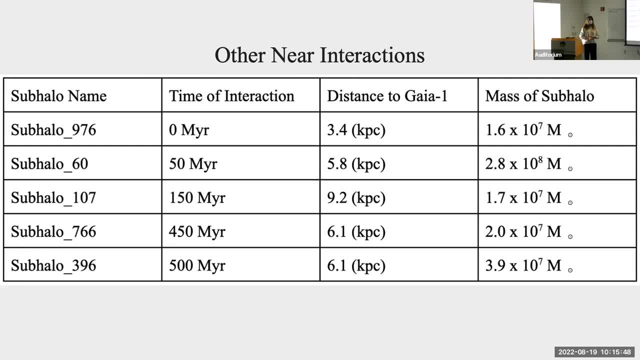 contact with, in the present and in the past, any other questions. so you mentioned that Gaia-1 was one of the streams that you were able to get in contact with, and this is a question for you. so is there a reason why you chose Gaia-1 and why exactly is the most useful stream to study? 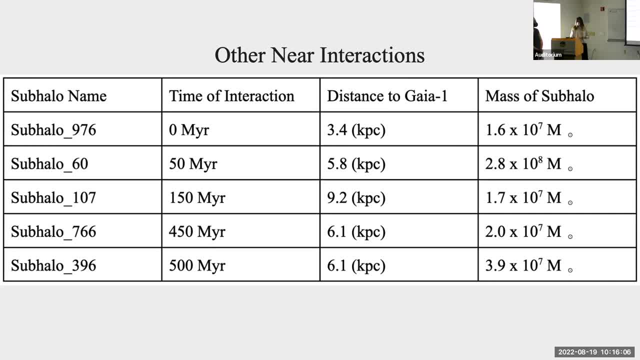 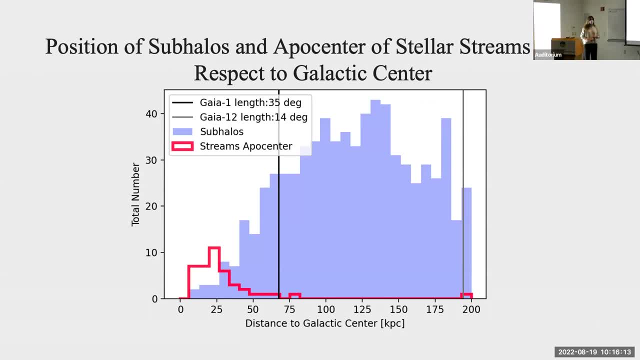 yes, all right. yeah, so I ended up selecting Gaia-1 due to its position in the sky, but also the epicenter. Gaia-1 was one of the one of the stellar streams that contained a larger epicenter and, as you can see here, I also did label Gaia-12, which had a larger epicenter as well. 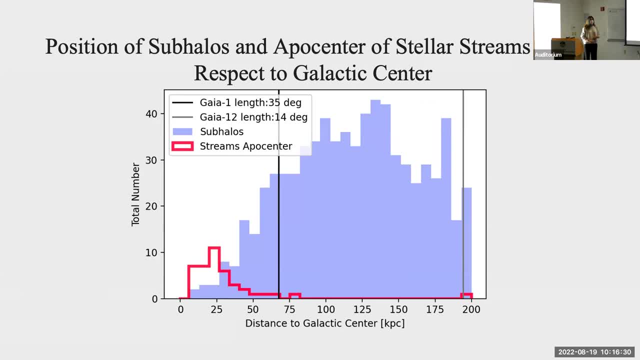 center with respect to all the other stellar streams. the main reason why we didn't decide on going with gaia 12 was because of its length. so its length is relatively short, of 14 degrees compared to gaia ones of 35 degrees. so we did want a longer stream, but also one that had a 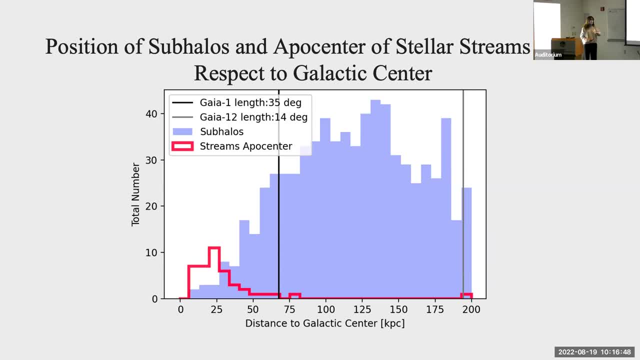 large epicenter, meaning that it could have gone further away from the center of the galaxy and closer to this region where the dark matter subhalos could potentially lie. great any other questions? all right, this will be the last one. so at the beginning of your presentation, you 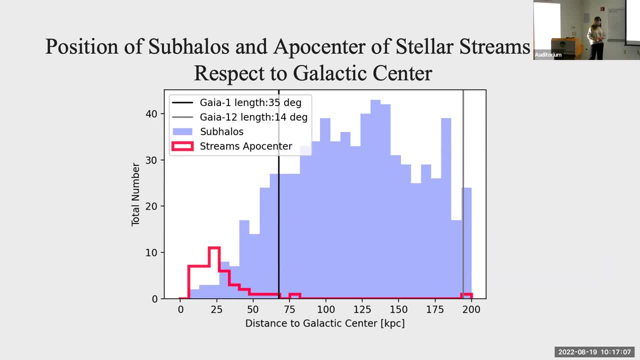 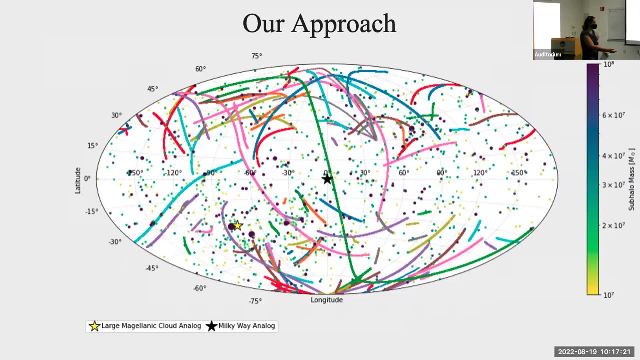 mentioned around about a thousand dark matter subhalos. i was just wondering if you could maybe talk about where that number comes from, if it's maybe based on observations or simulations. yes, so for our dark matter subhalos, the actual um simulation was was ran by ethan nadler. um, there was much more dark matter subhalos that could theoretically 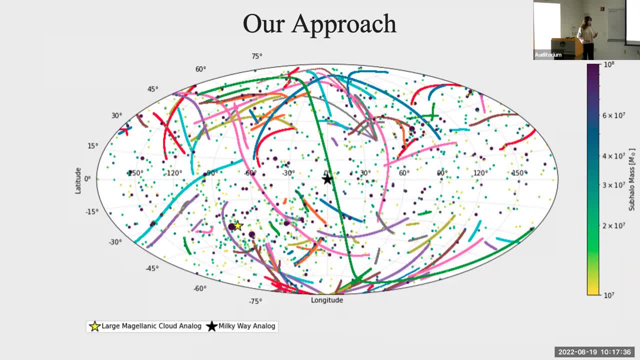 exist in our galaxy. however, i ended up having left 1072 of them simply because i added the constraint of a mass greater than 10 of the seven solar masses. so there were more of lower mass, but in order to make it more credible and have a higher chance of having a greater impact and